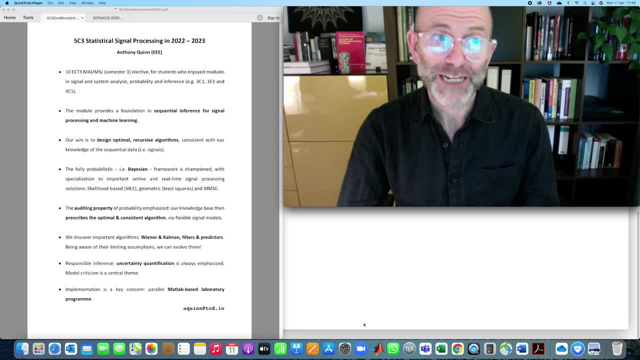 certainly appeal to students who have had an interest in signal and system analysis, in probability and inference techniques, modules such as 3C1, 3E3 and 4C5. but I very regularly welcome students from other areas of the university and indeed many of our visiting. 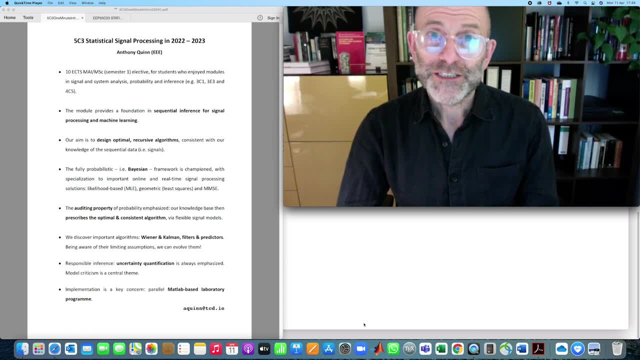 students as well. So the module is concerned with design principles for recursive or online signal processing and also addresses some key paradigm problems in machine learning, And our concern really is that the design of these algorithms be consistent with our knowledge of how the data were generated in the first place, the context in which we are 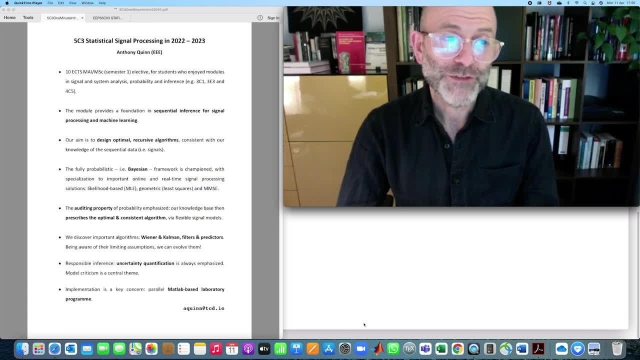 undertaking our algorithmic design. So for this purpose I champion the fully probabilistic approach to the quantification and manipulation of uncertainty, what we call the Bayesian approach. But we're careful, amid that universal framework, to specialise to some of the really important classical criteria for the design of some very important algorithms in signal. 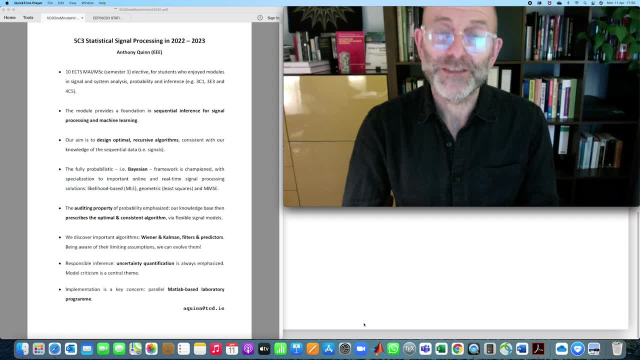 processing, likelihood based approaches, maximum likelihood estimation, geometric approaches, least squares estimation and the minimum mean squared error criterion of Wiener for optimal filter design. But this Bayesian approach is important in providing us with an auditing framework which essentially forces us to travel through all the assumptions. 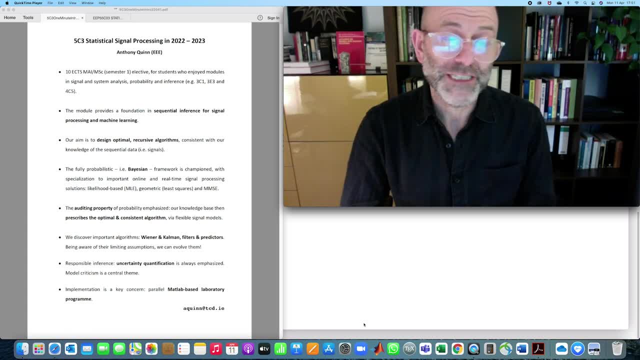 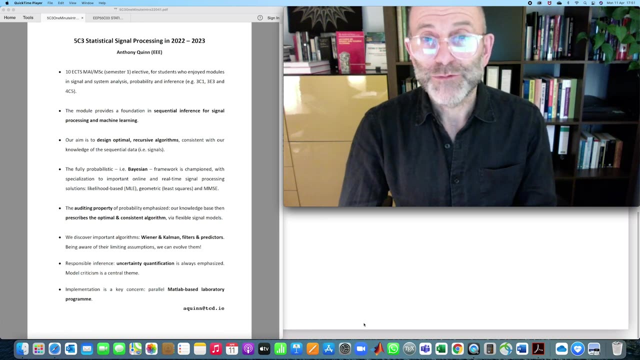 that we are making about the data sets that we're studying And then, in many ways, non-optionally, if you like- in a prescriptive pathway. this leads to algorithmic design that has optimality properties and consistency properties, And we lean heavily on very flexible model structures. 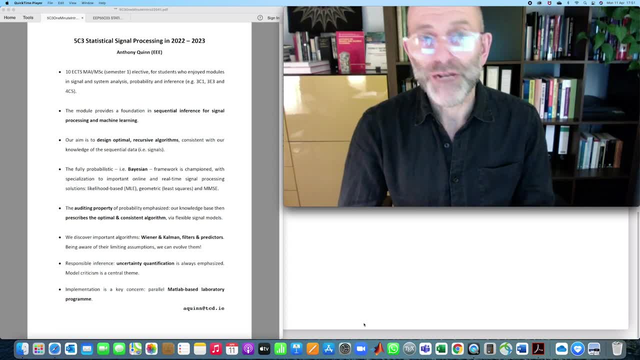 models that can be applied very widely, notably linear regression structures and various autoregressive structures. And along this pathway we encounter some of the really important algorithms that have been implemented in practice and, as I say, very widely across applications: The Wiener 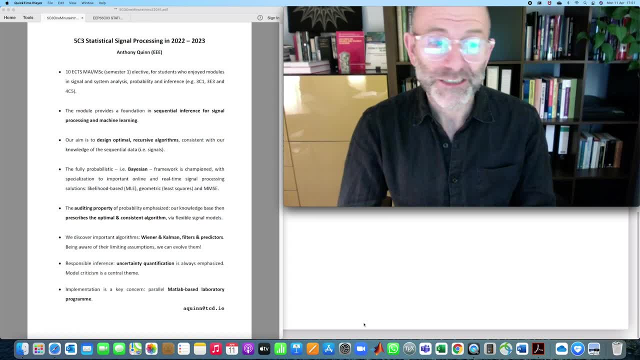 filter and the Kalman filter and their various predictor variants, And in understanding them in this Bayesian framework, we also become aware of their limitations and the limiting assumptions under which they were designed. And in some ways this is an invitation to evolve them, sort of a research invitation, as is appropriate, I suppose, for a